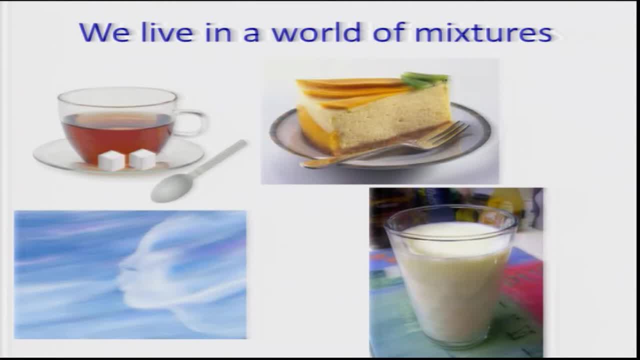 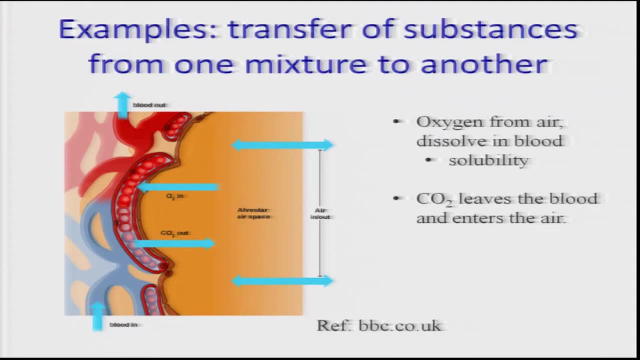 or, for example, the milk we drink And its separation, stability, transfer for one species from one phase to another is of direct importance to many applications, including what I just showed. So we will take some examples, typically, which are important for sustainability of life. 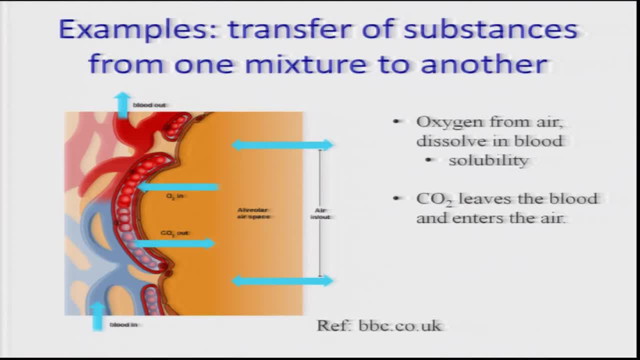 First one is we are talking about how a mixture after the transition, its solution in blood and if you see, here the oxygen from air gets dissolved in blood and it depends on its solubility, that is, how much it can absorb oxygen from air. In the process, the CO2 also leaves the 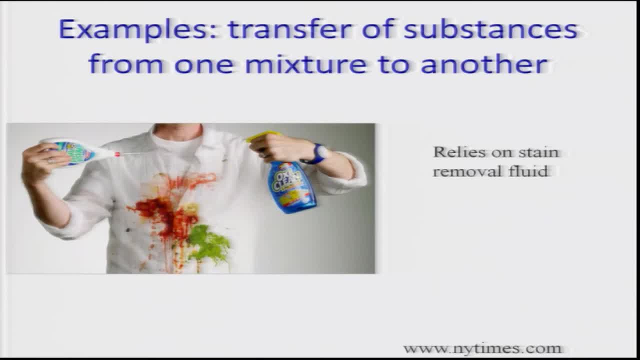 blood and enters the air. This is an example of transfer from substances from one mixture to another. Here is another example. This is basically again depends on the transfer of substances- for example, your shed- and it depends on how much affinity of this stain for the, this fluids. 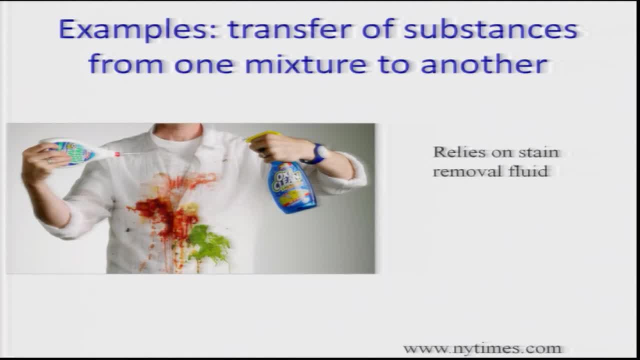 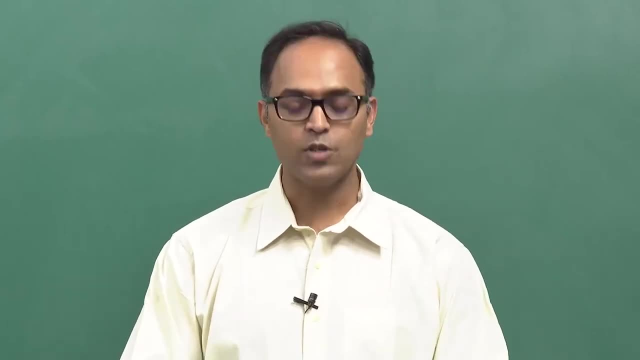 which you use. okay. So, in other word, the fluid which is you using in order to remove should have high affinity or, in other word, high solubility. So, in one sense, the idea of transfer from one phase to another and, in other word, the 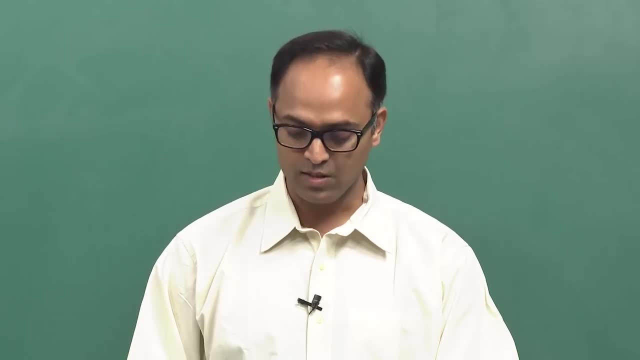 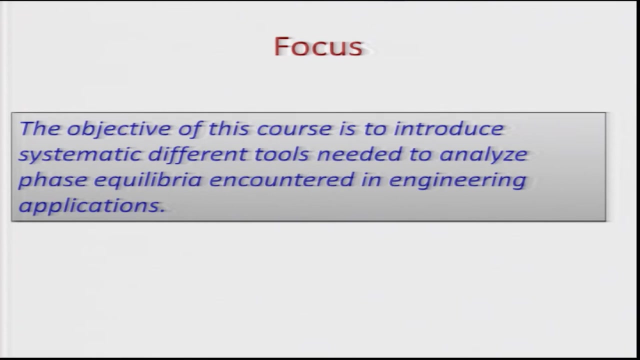 mixtures, as phase stability and in different phases, are of direct importance to applications and we will be taking such examples in this course. okay, So our focus would be to introduce systematic, different tools needed to analyze phase equilibria encountered in engineering applications. So that will be the focus of this course. 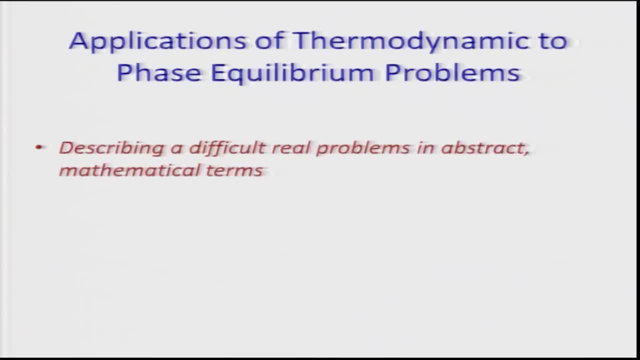 In the process we will be considering different applications- example of various different applications. We will be considering something in abstract form and we will be taking that abstract form and convert into the mathematical term. that is the first step of analyzing the problem in using thermodynamic tools. okay, 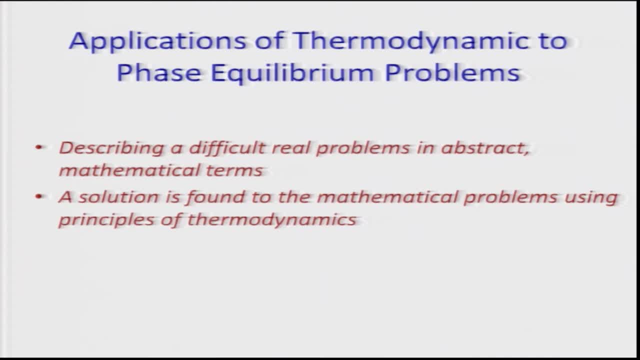 The second thing is we are going to do is the solution will be try to find it using mathematical, in mathematical problems. okay, using the principle of thermodynamics, okay, So a solution is found to the mathematical problems which we going to describe, the problem statement: using principle of thermodynamics. 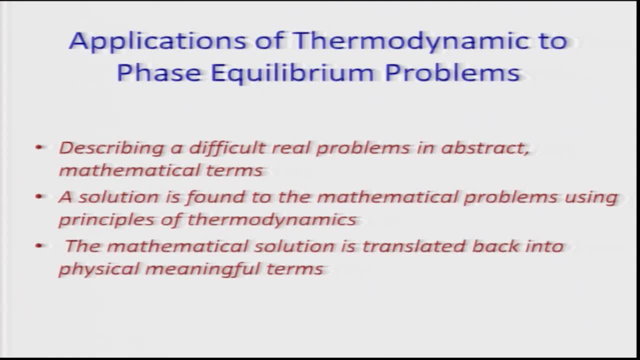 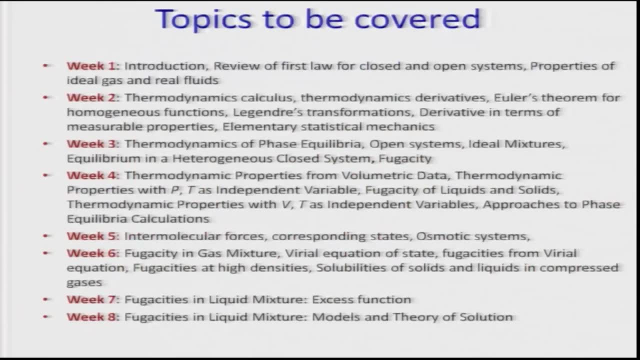 And the third is the mathematical problem And the mathematical solution is translated back into the physical, meaningful term. So this is the kind of a steps which you are going to take in this course, okay, And the detail, the topics which we are going to cover, is given here in the first few weeks. 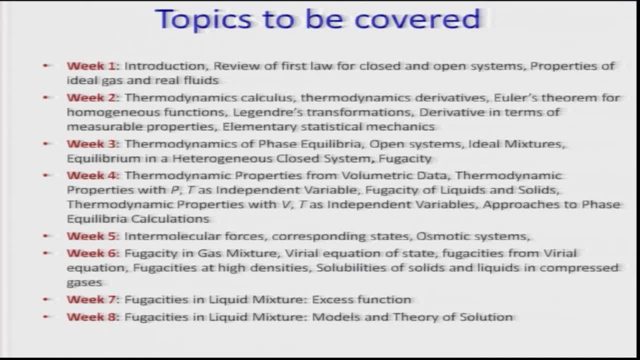 we are going to cover the introduction and the basic thermodynamics, essentially to have the foundation for taking up more complex problems. So if you have done the engineering thermodynamics in your undergraduate, you should be able to take it, irrespective of if you have taken the chemical engineering. 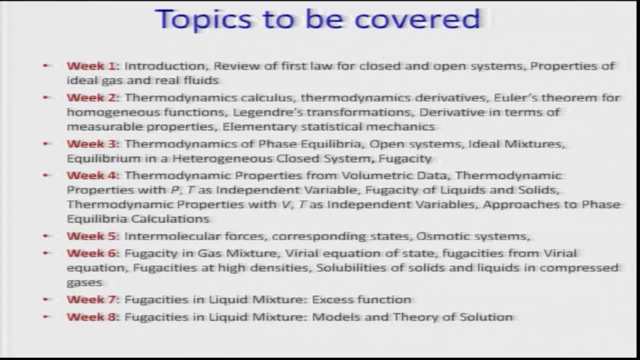 So this is the kind of a steps which you are going to take in this course. okay, and the chemical engineering thermodynamics, not, because certain introduction will be given so that you can take up the problem of challenging type. okay, In the week 3 we will start the thermodynamics of phase equilibria: open system, ideal mixtures. 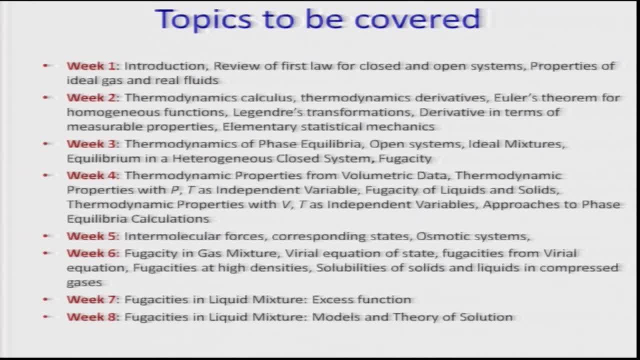 and equilibria with the heterogeneous closed systems and we will introduce something called fugacity And in week 4 we will try to evaluate properties of thermodynamics using volumetric data. okay, and define fugacities of liquids and solids which you are going to use in the next class. 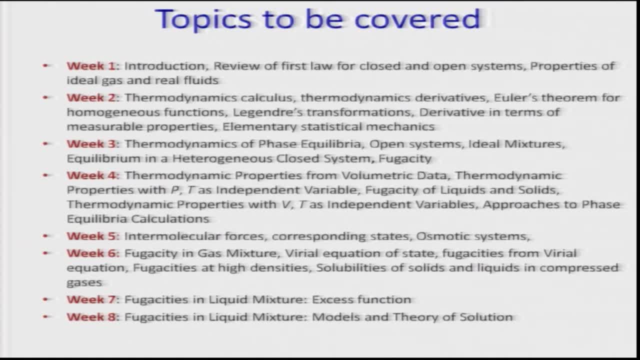 So we are going to talk about the properties of thermodynamics using volumetric data, okay, and define fugacities of liquids and solids, which you are going to use in the next class, Okay, So we will go a little bit later for phase equilibria calculations. 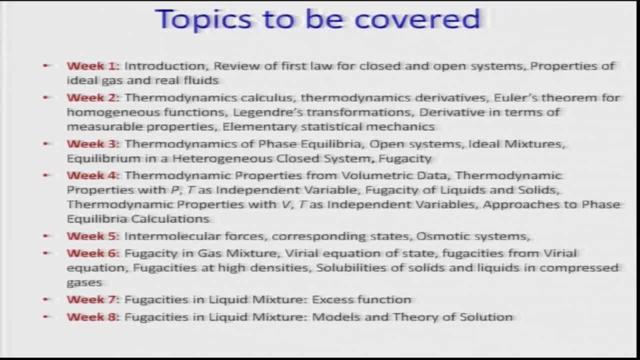 In week 5 we are going to define the forces responsible for many of this phase equilibria, and week 6 we will go through the fugacities, gas mixtures, virile equational states. okay, fugacity as a high density and solubility of solids and liquids in compressed gases. 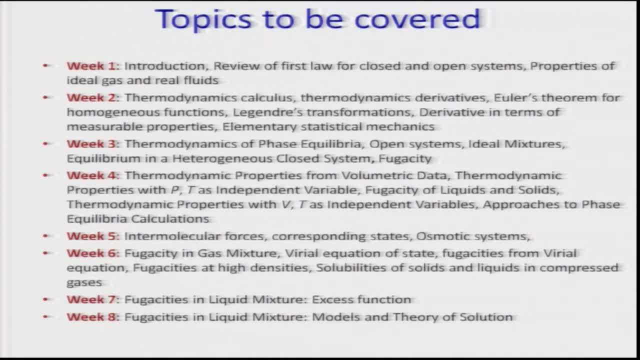 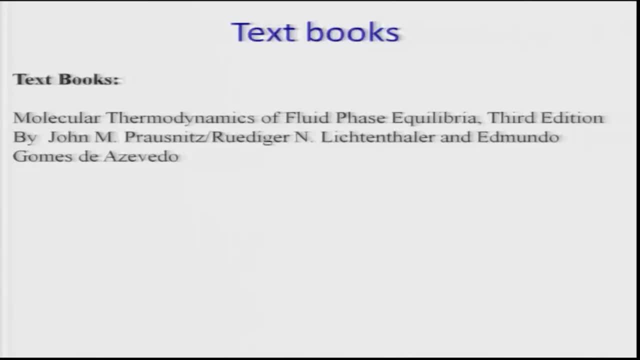 And week 7 and 8 will be looking into fugacities, liquid mixtures, in more details. okay, So that will be the topics which we are going to cover. Okay, So the next test book which we are going to follow is molecular thermodynamics of fluid. 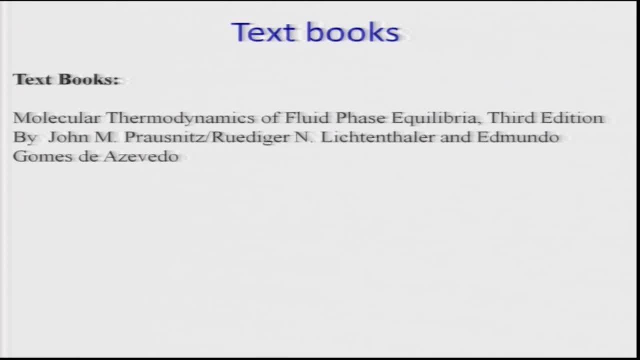 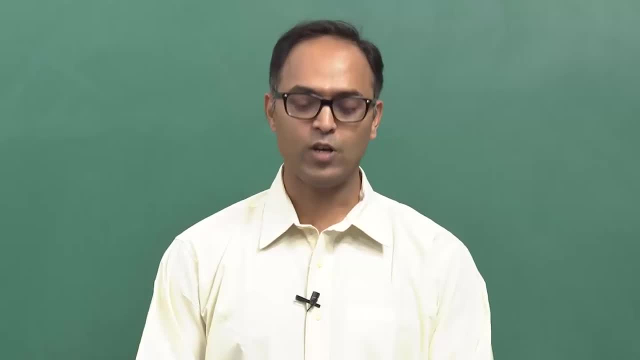 phase equilibria, third edition by Proznes and co-authors. There are many other test book which one can refer, but this is the main test book which we are going to follow. The notes will be provided, So I hope that you are going to like this course and join us to enjoy the thermodynamics.